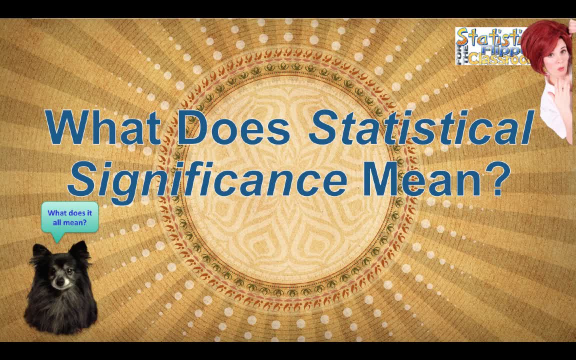 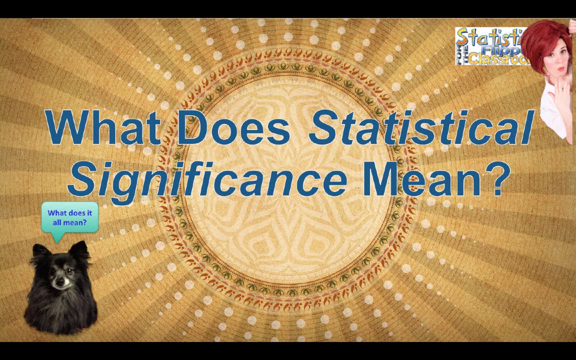 It is very important that we understand what is meant by the phrase statistically significant difference. We know that significance is indicated by a p-value less than 0.05, but before you go getting all excited about the size of your outcomes p-value, let's be clear about what significance really means. 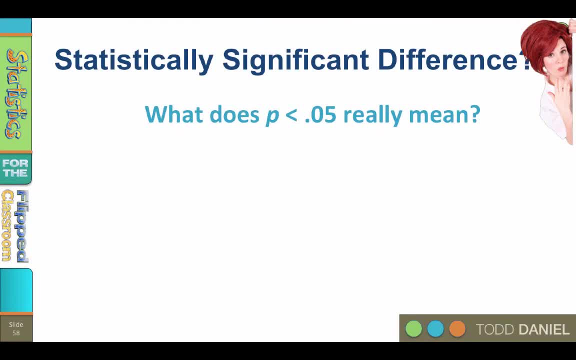 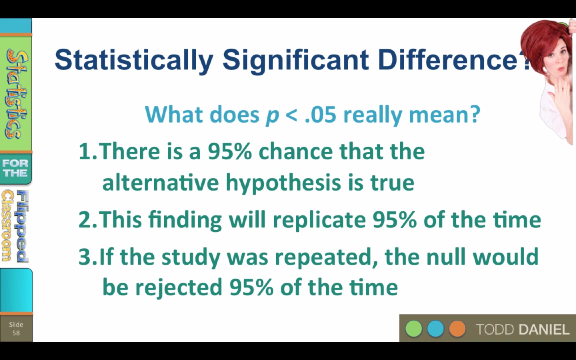 When you find a statistically significant difference, does that mean that there is a 95% chance that the alternative hypothesis is true, Or that this finding will replicate 95% of the time, Or that, if the study was repeated, the null hypothesis would be rejected 95% of the time? No, 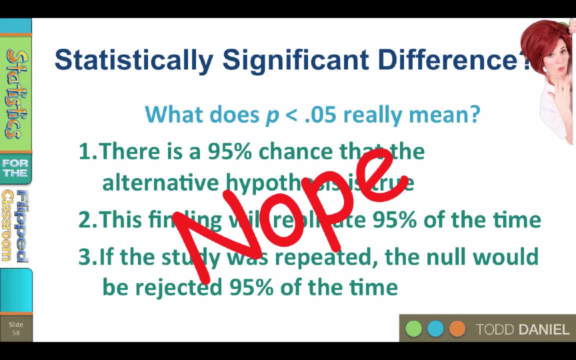 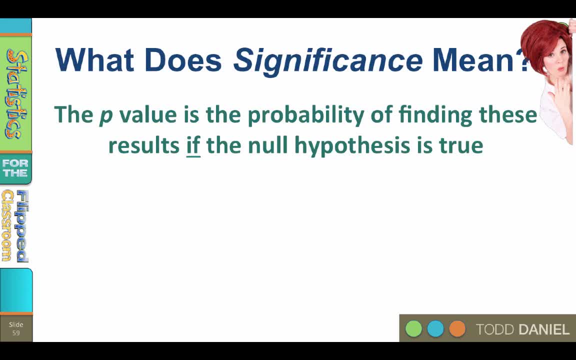 It means that the null hypothesis is true. It means none of those things. So what does p less than 0.05 really mean? The p-value is the probability of finding these results. if the null hypothesis is true, A statistically significant difference- p less than 0.05,- means that 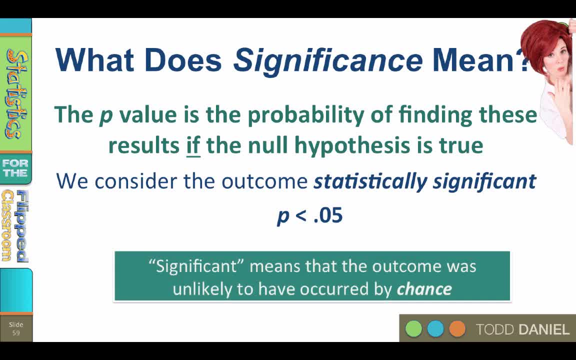 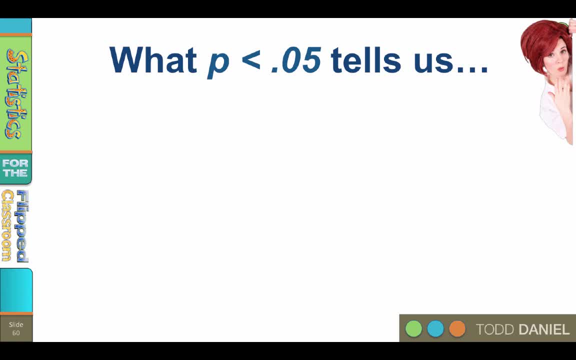 the outcome that we observed was unlikely to have occurred by chance. What p less than 0.05 actually tells us is that the results were statistically significant, but it does not tell us whether the results are practically significant. In other words, do these results really matter in the 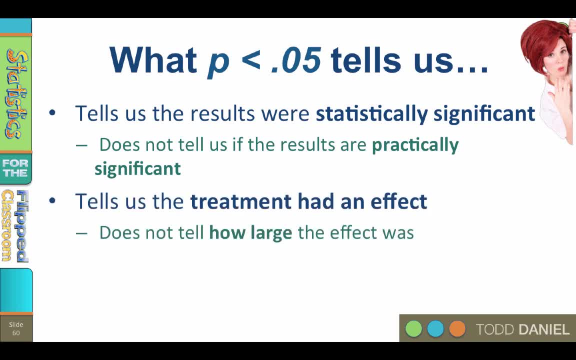 real world Statistical significance tells us that the treatment had an effect most likely, but it does not tell us how large that effect was. And finding a p-value that is very small- say less than 0.001, does not make the results quote more significant. There is no such thing as being more. 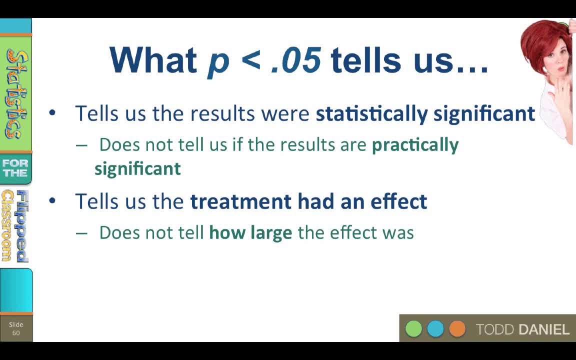 significant. The results are either statistically significant or they are not. In order to know how large the effect was, we need a measure of effect size. So we may have found an effect, but the effect was really small and of no real-world importance. Measures of effect size will be things like Cohen's. 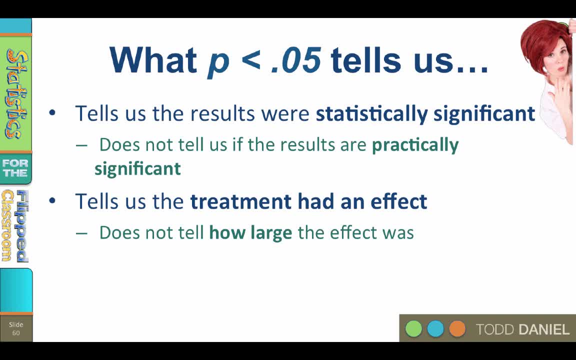 d? r-squared and eta-squared. Statistical significance tells us to reject the null hypothesis, but it does not prove that the alternative hypothesis is correct. Whenever we make a decision, we could make a mistake. As we learn more about hypothesis testing, it will be important that we not rely 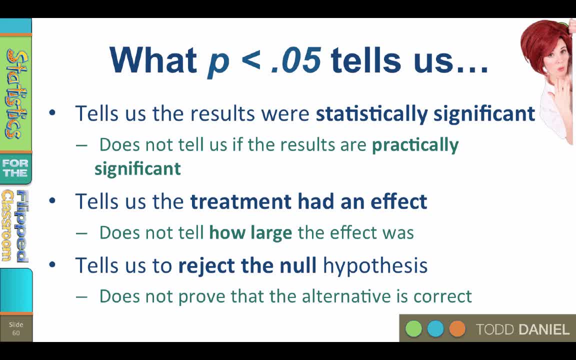 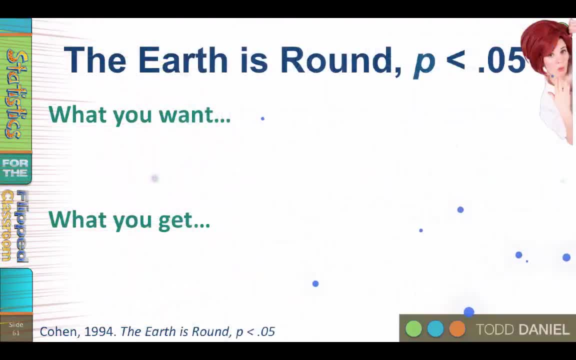 exclusively on p-values, but also consider things like effect size, confidence intervals and the power of our test. We need to think about what Jacob Cohen wrote in an article titled The Earth is Round. What you want to know when you do hypothesis testing is the probability that the 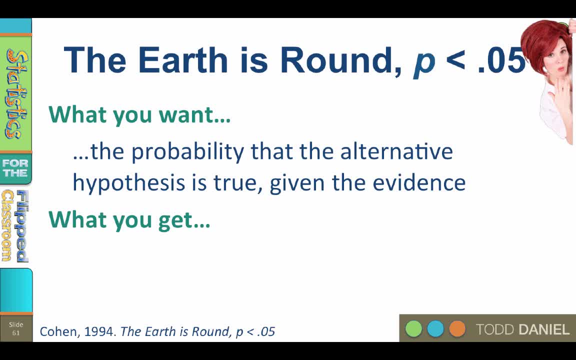 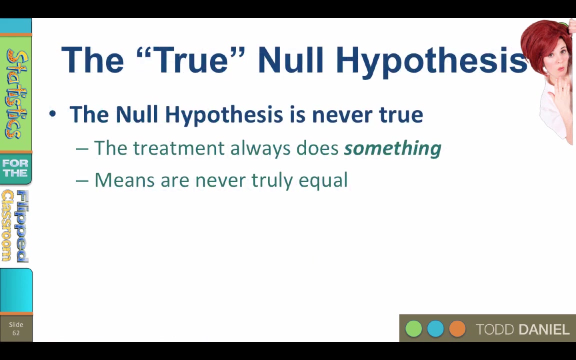 alternative hypothesis is true, given the evidence, Did the treatment have an effect? What you get, however, is the probability of obtaining this evidence, assuming that the null hypothesis is true. If the treatment really did work, then how likely is it that we would have found these results? Well, the big problem. 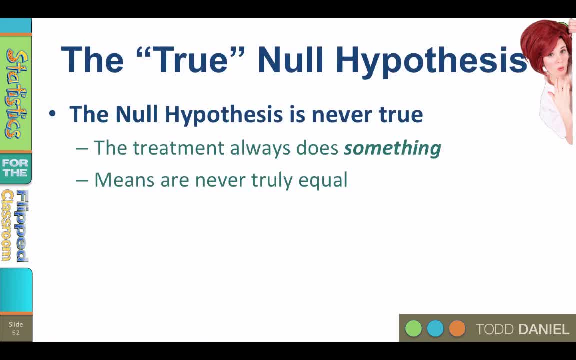 with this approach is that in reality, the treatment always works. It always does something, even if that something is trivial And means are never truly equal. If you go out enough decimal places, they will diverge. So the null hypothesis is never actually true, Furthermore improbable. 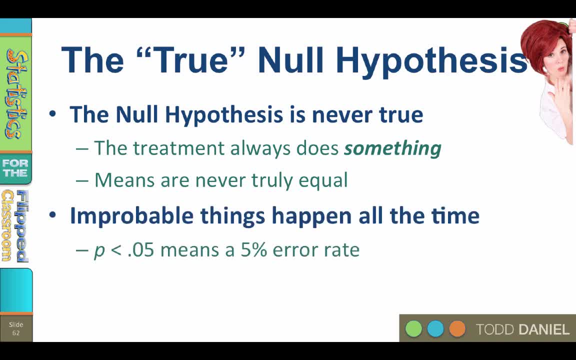 things happen all the time. In fact, if you do enough tests with the same ineffective treatment, some of those means will in fact be statistically significantly different. p less than .05 means that five times out of 100, one time out of 20, we will. 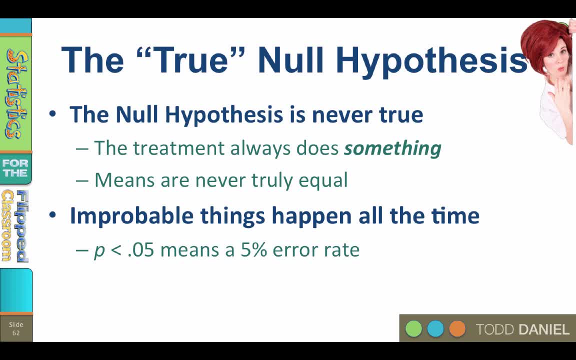 make a mistake. We will mistakenly identify an effect as significant when in reality it's not. We make a type 1 error. This is also called the dance of the p values. And finally, statistical significance is a function of sample size. With enough people?